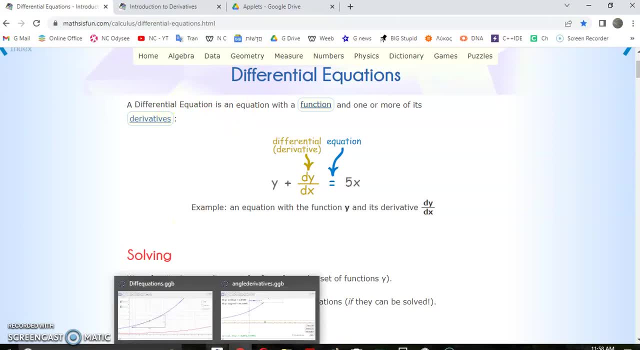 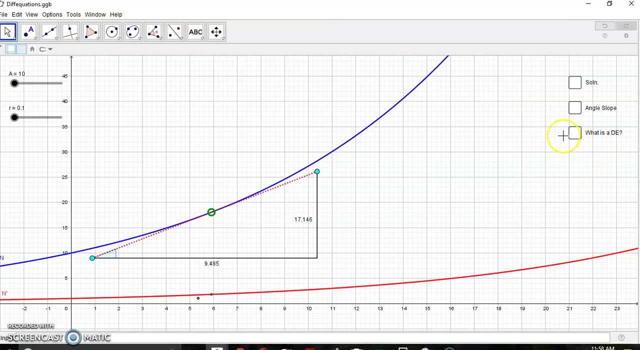 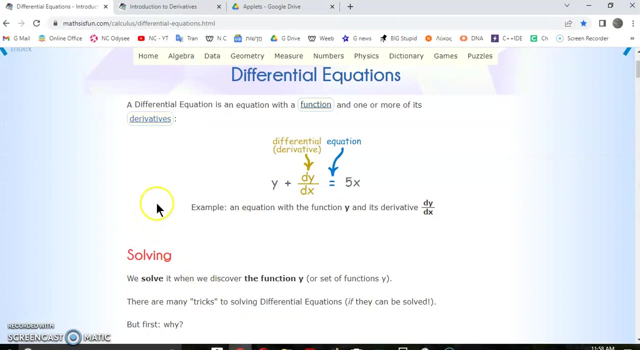 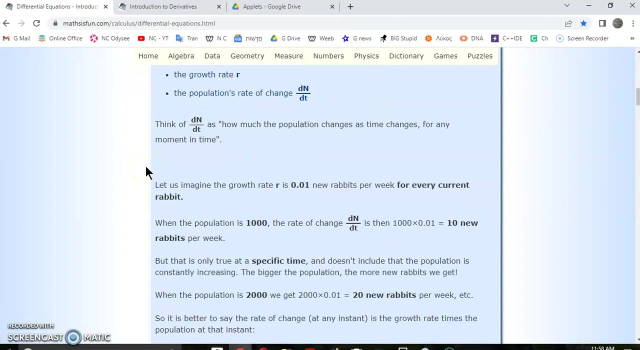 So this definition here is not really a very nice one, but I'll get back to it shortly and I'll show you exactly what the definition is and then proceed to give you a little demonstration here of all these things. So this site here tries to give you an example of how we use differential equations, and the most common is the one with the. 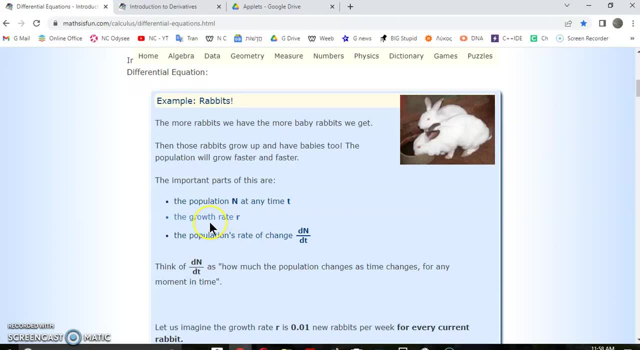 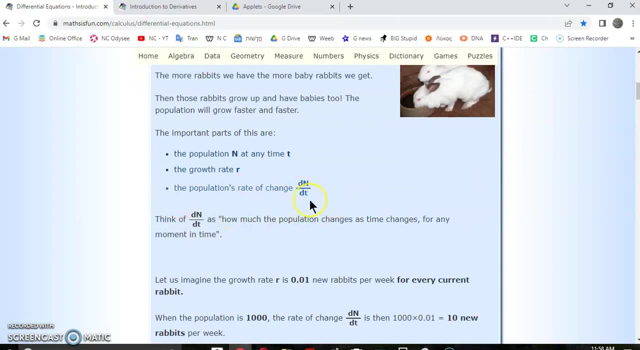 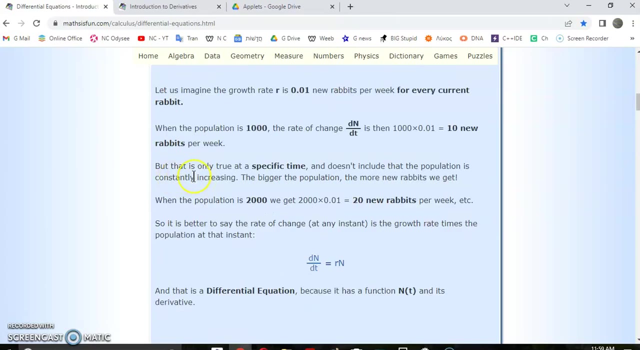 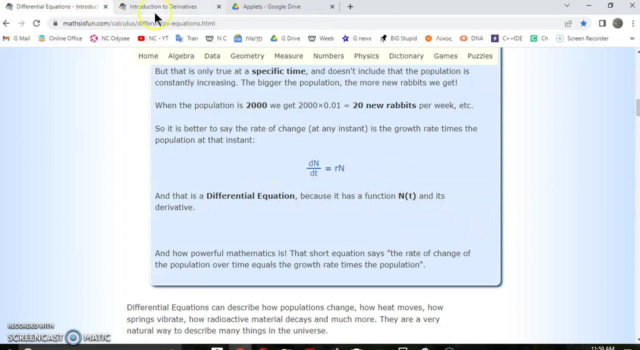 population expressed as a function of time. So, and normally in any such equations, we always have the exponential function, the natural exponential function, which is E, which is known as E. Okay, so it's the constant E And that's pretty much what this site says, and because it's not important, I'm going to close it. 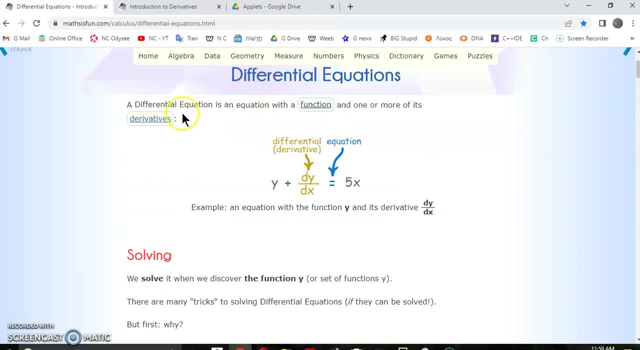 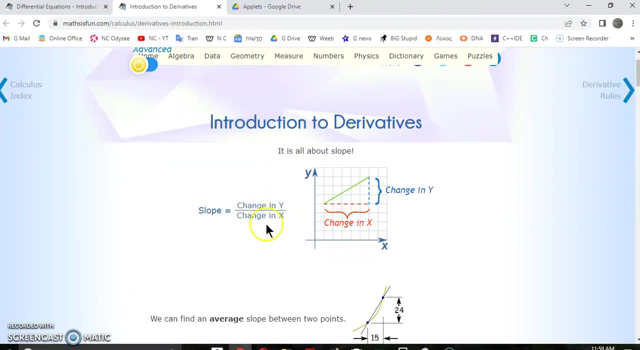 There's one other problem here. In this definition it says one or more of its derivatives, but if you go to the link, a derivative has nothing to do with change in anything. So this definition here, which is ubiquitous in the mainstream, is actually wrong. 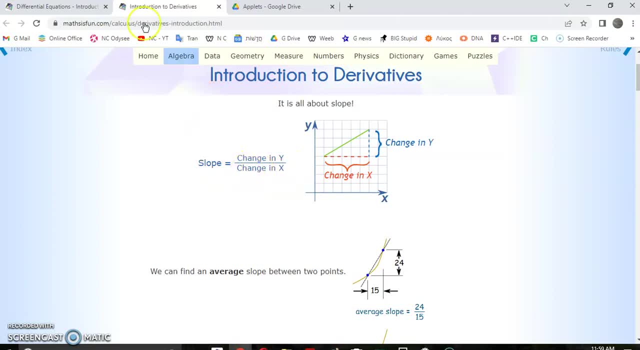 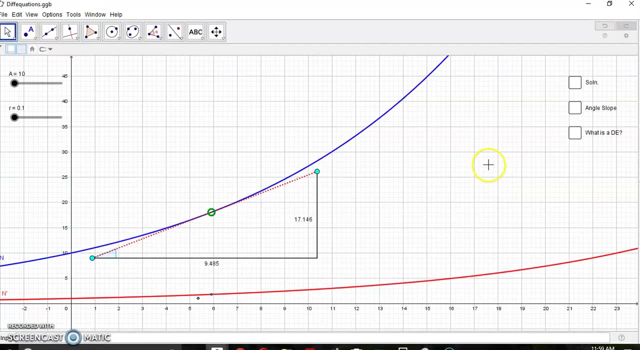 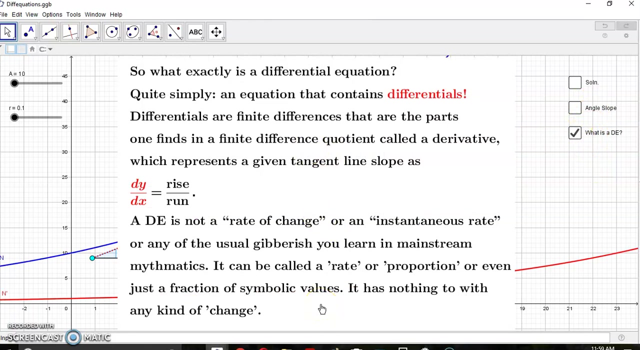 Nothing actually changes at any time ever. So let's close that, get it out of the way and and look at what is the differential equation. So I suppose that, quite simply- and it's a differential equation- is an equation that contains differentials. So what are differentials? There are finite differences that are parts. 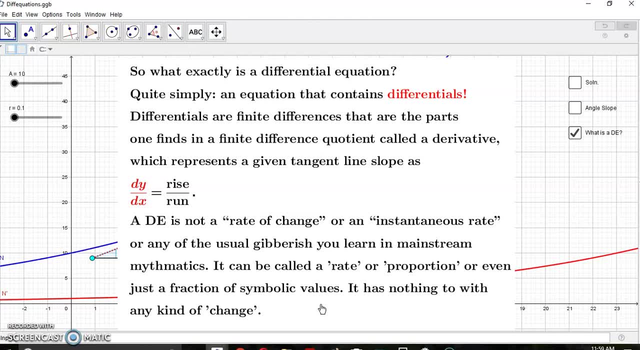 There are parts one finds in a finite difference quotient. Okay, so the finite differences do not change right, There's nothing about change there, And they're basically the parts one finds in a finite difference quotient, which we call a derivative, And 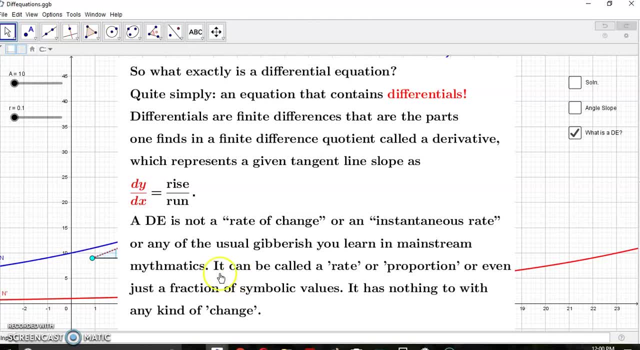 it represents a given tangent line slope as rise over run, as you see over here. So dy and dx are examples of differentials. They're just finite differences, right? Not a change in y but a change in x, Just a finite difference. 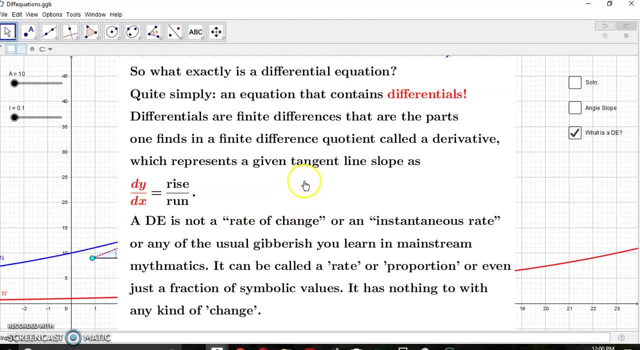 Because the y's and the x's for any given smooth function haven't changed in past probabilities And they're not changing in future perpetuity- future perpetuity either. So a differential equation is not a rate of change or an instantaneous rate or any of the usual gibberish you learn in mainstream. 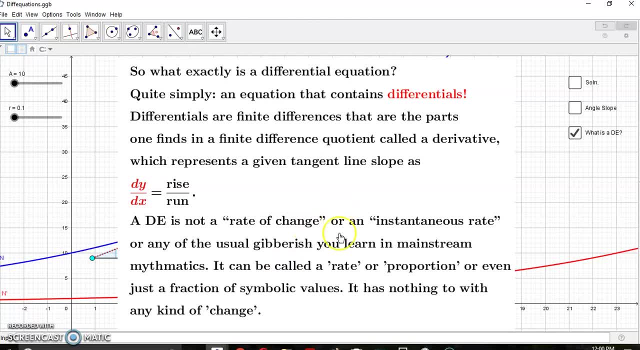 mathematics. Okay, so it's really just. it can be called a rate or a proportion, or even just a fraction of symbolic values. It has nothing to do with any kind of change, But in order to pass on your exams, you need to understand how to relate this gibberish to what is actually meant in reality. 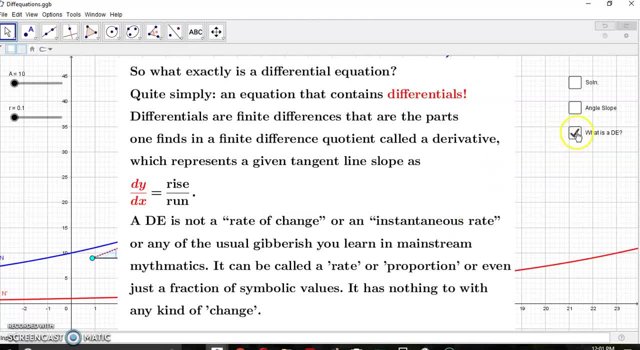 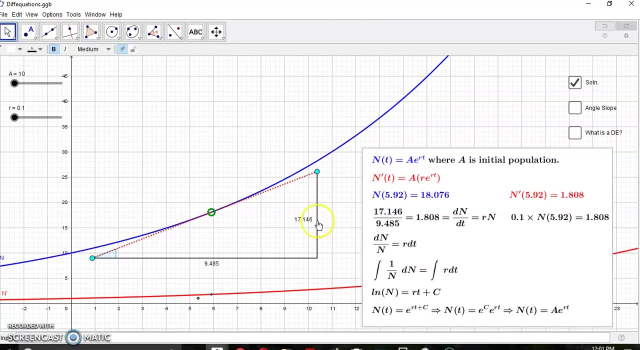 and I'm not going to do that in this video, because I've done it in many other videos and I've also explained what are differentials in previous videos. I encourage you to go and watch those videos. So the example that one looked at on that website is natural growth, So this is normally. 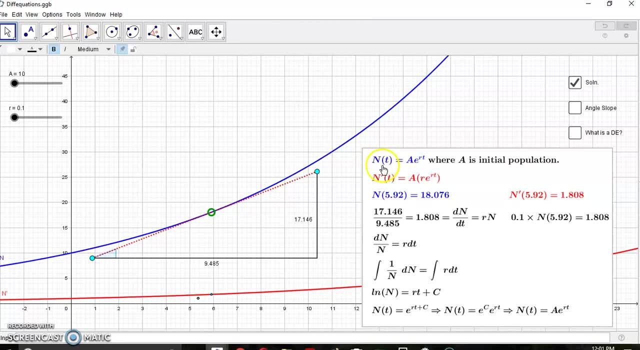 expressed as a function of time. so n would be the number of people in the population and a would be the initial population, and this would be the function that is expressed in terms of time. So nt is a function of time and its derivative, this red curve, is also a function. 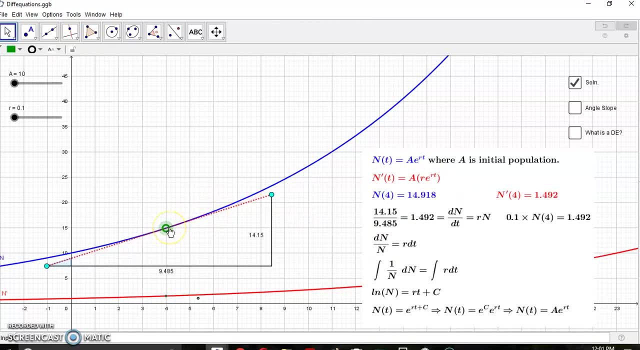 of time and we can see that all that dn, dt is is just the slope of this tangent line at any given point. okay, it doesn't change. So these are the finite differences. by the way, 10.884 over 7.296. okay, those are dy and dx exactly, At least in the new calculus. these 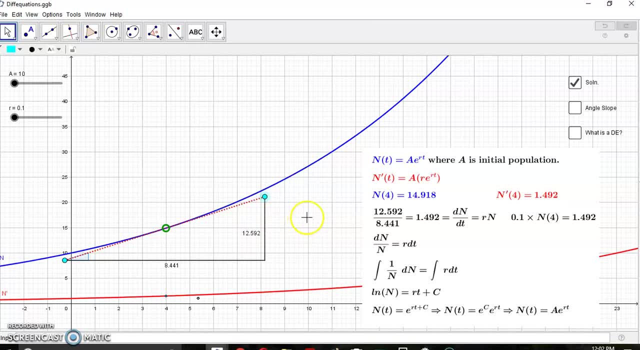 work exactly in your bogus calculus you've got the problem of limits, but when I'm not going to talk about that either, because I've talked about it in previous videos. So what mainstream academics do is they take this function here, which you see dn, or 1 over n times dn, because that's. 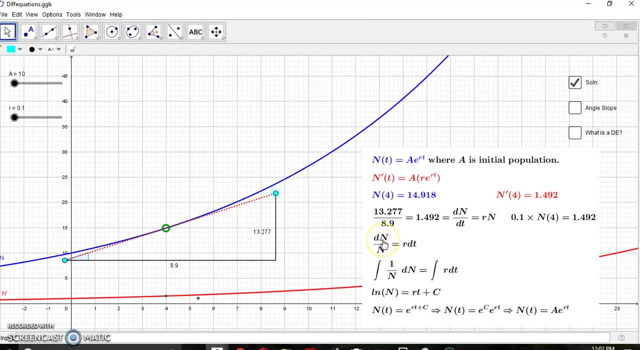 exactly what we're going to do. So what we're going to do is we're going to take this function here, which you see, dn, or 1 over n times dn, because that's exactly what that means and, yes, dn is a symbolic value, is equal to r, which is the supposed growth rate. 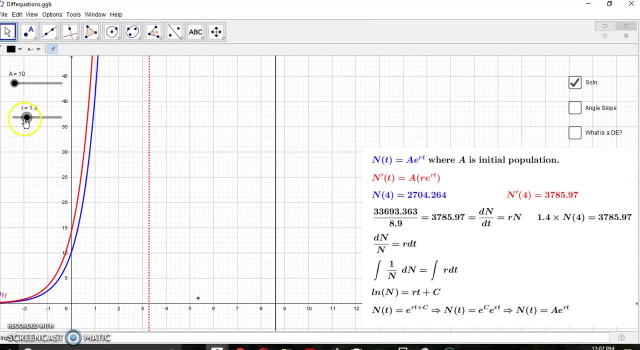 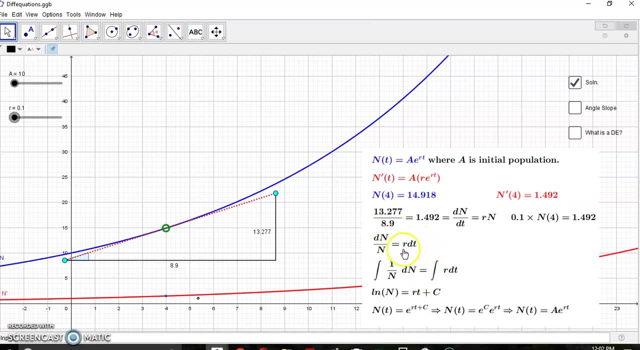 It's just some constant like 0.1 or something else, and multiply it by the differential dt. So in this case, because dt is a differential involving time, one might think of it as a rate of change, but it's strictly true, Strictly speaking, not a rate of change, because it still belongs to this function. n of t is equal to. 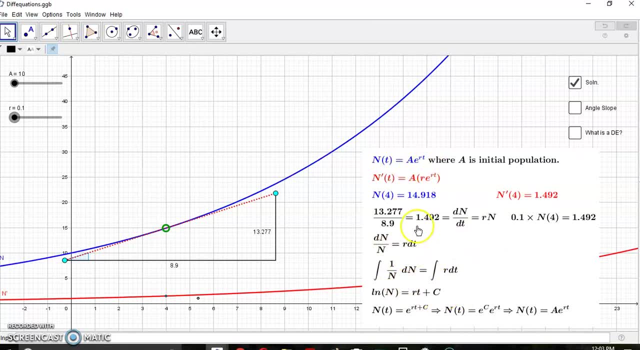 a, e to the rt. So to solve this, in order to find an original function, if we don't have n of t and we're just given the differential equation, we integrate first of all. this integration process is the most common. it's called separation of variables. It's the one you'll love the most. 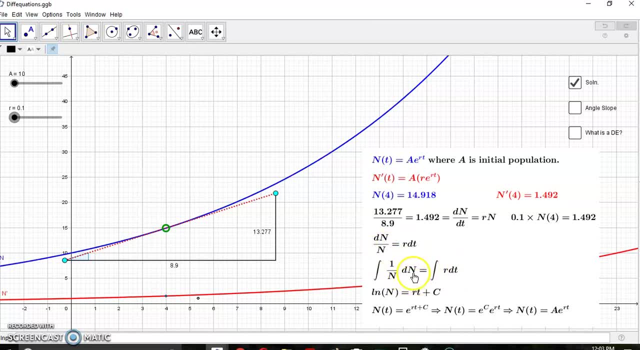 because it's the easiest. So you, you, you simply take the original differential equation, which is: dn, dt is equal to r. okay, in other words, this one is equal to rn, dn, dt is equal to rn, and you multiply, you divide both sides by n and multiply both sides by dt, just as you would values, and then you integrate both sides. 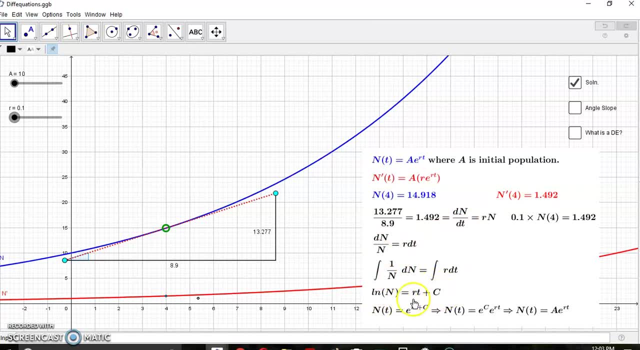 and by so doing you end up with the logarithm of n is equal to rt plus c, which, of course, if you rearrange this or take both sides to base e, then you have the original expression of the function in terms of time, which is equal to e to the rt plus c, and of course this here is also equal to. 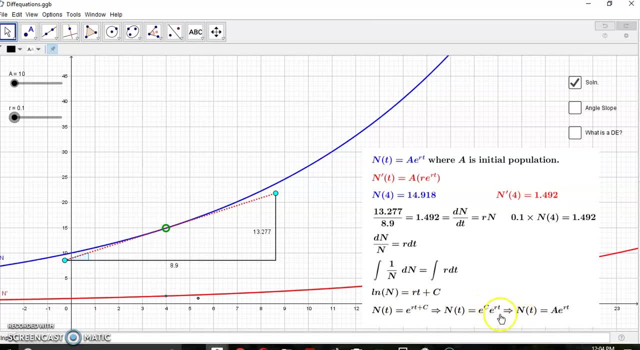 e to the c times, e to the rt, meaning that we can just say that e to the c is some constant and we'll call that constant the initial population. So that's all they basically do as far as this is concerned. okay, and when you move this point along on the original function, you'll see that. 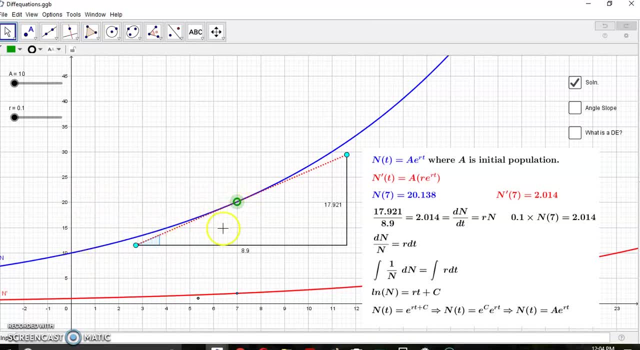 it gives you the approximate value of the population. So if we started at time zero, we have 10, and if we move to time t, equal to t7, we have approximately 20. we have 20 individuals, because you can't have a fraction of a an individual. okay, So that's pretty much it. 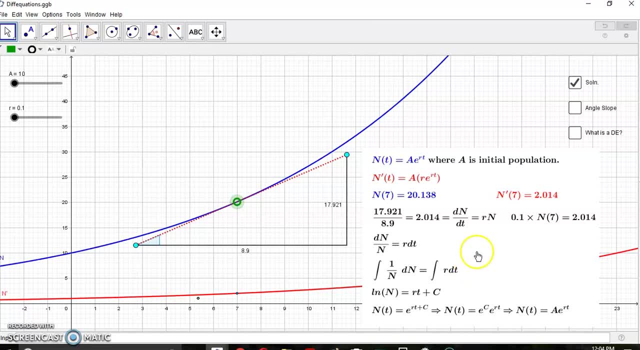 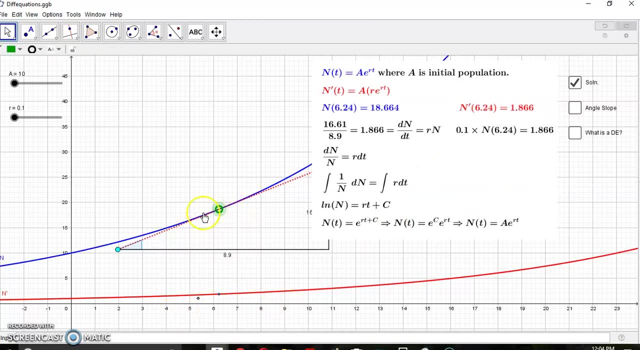 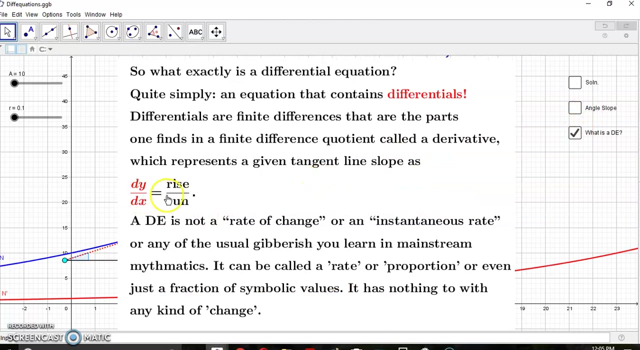 as far as the explanation goes, and now you know, a lot of emphasis is placed on finding the derivatives and you think, wow, so do all these values. they go on to become innumerably many. but if you had to consider this in terms of angle slope and not rise over run, so if, for example, dy to dx was expressed, 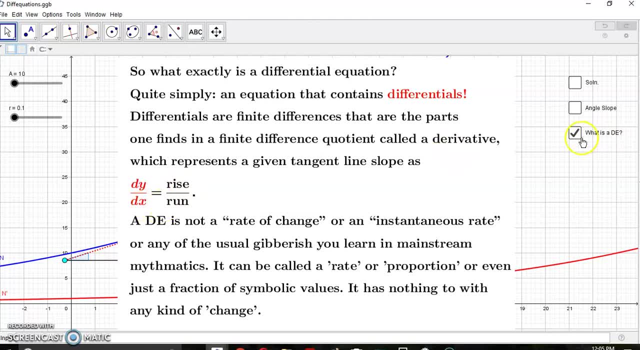 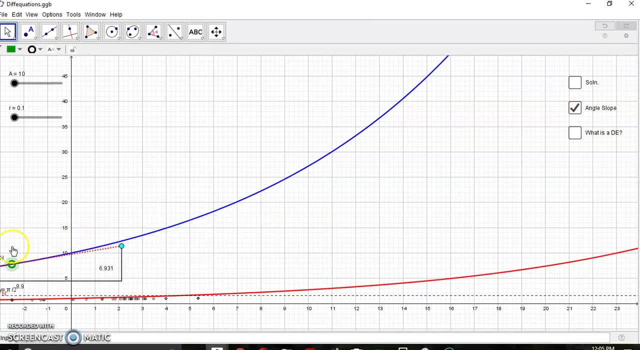 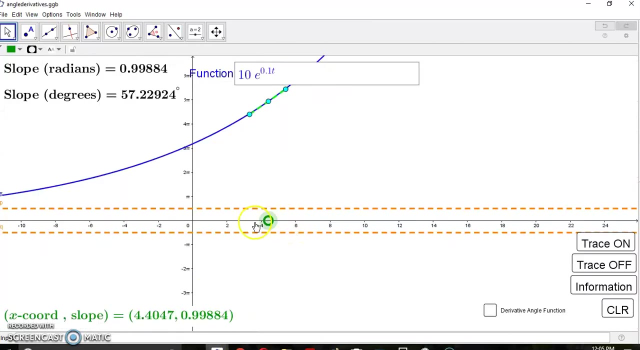 as a function of angle slope, then really, what you'd have is, if you move it anywhere along the side, you'd have a function whose range always falls between pi over 2 and minus pi over 2, and in this case it's 0 and pi over 2. okay, so in this case you have the special function where, if you move it anywhere, 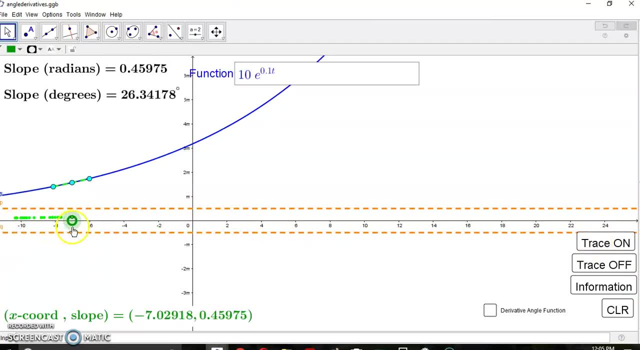 let's put the trace on. so if you move this anywhere along here to find the derivative, it always lies between y equals 0 and y equal to pi over 2. okay, so it's always inside here all the way up to 0 and it's return on net term. so here we have. we're left with 1. we can't test this. 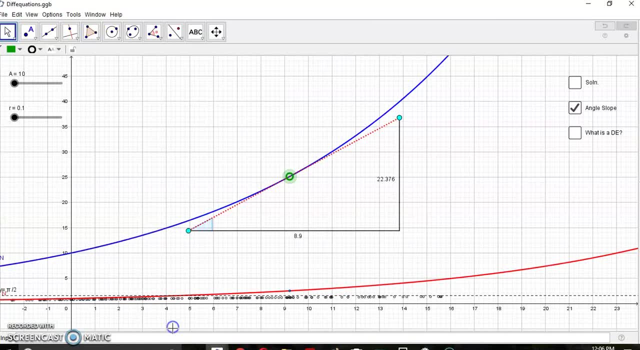 right away. we're going to solve just Beckmann's equation. does it give us an axis in the derivative to find the derivative? sorry, he, he tells you the definition. uh, and if you're looking at the diagram you'd find the equations are different. so you'd have to try and comprehensively compare the dia set up. so let's find out if it will fit in the 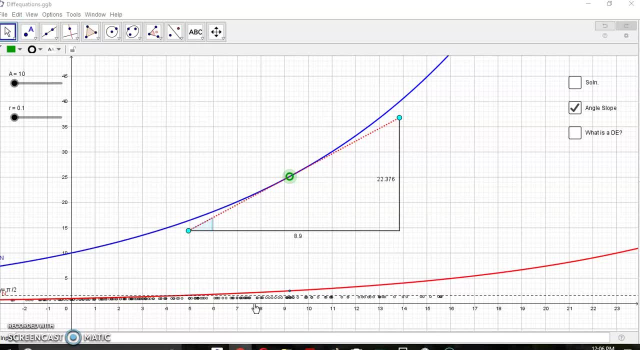 function. it talks about a differential function as containing one of its derivatives, but it doesn't have to be a derivative of the function itself. It can be a derivative of any other function. It doesn't particularly have to be a derivative of that particular. 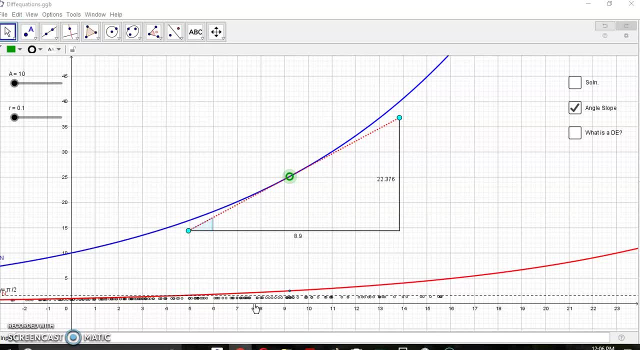 function. So as long as the y's were equal, then you'd have a valid differential equation. So also parts of the function can be expressed in the form of a second or third or fourth derivative. So you'd have an ordinary differential equation of a certain degree. So that's pretty. 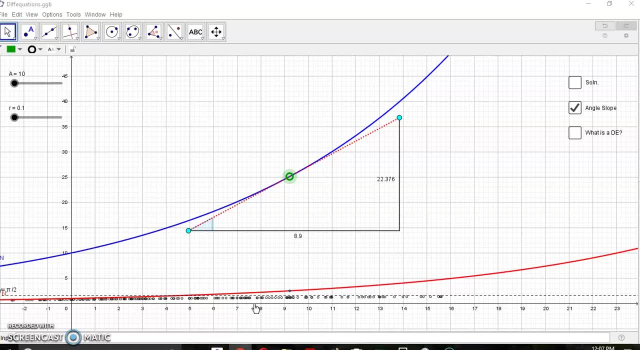 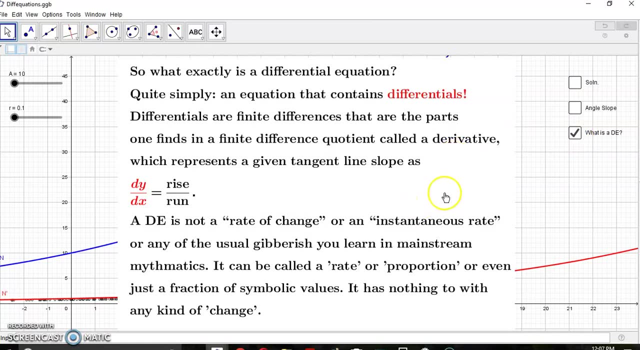 much it. I hope you've learned something from this and that you now understand what is DE. And just to recap, it's simply an equation that contains differential, at least differential. It contains two differentials, okay. It cannot contain one and it cannot contain an odd.